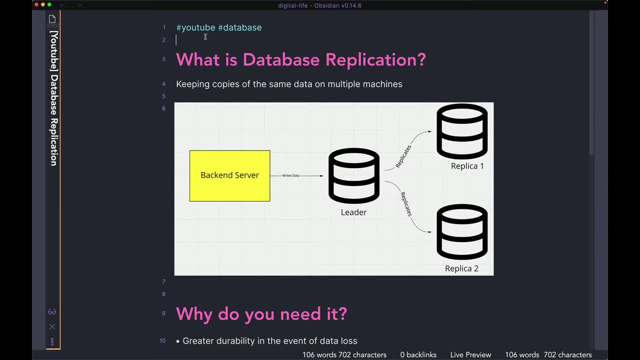 You have replica one, replica two and your backend server, which is the yellow box to your left, is writing the data to the leader database and the leader database is replicating the same data into replica one and replica two. What this means is you have essentially the same data. 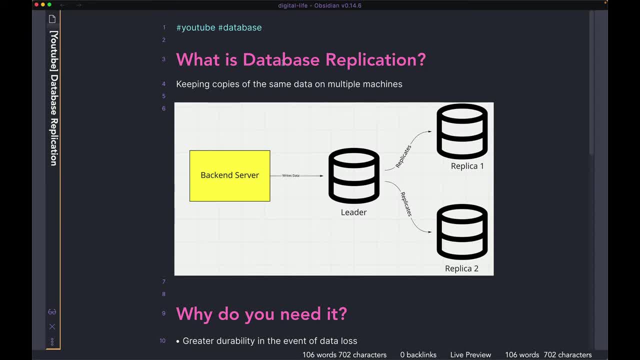 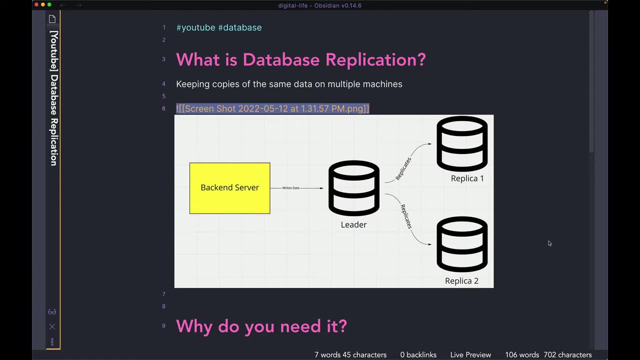 in three different machines. So the three you see over here, so one, two and three- all three are entirely different machines. So even if one of the machine is not working for some reason, you can stay confident that your data is safe in the other two machines. 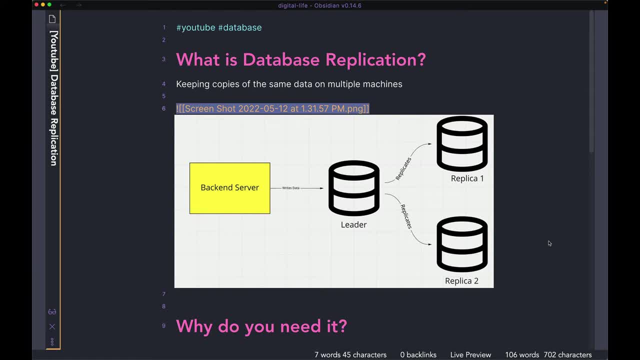 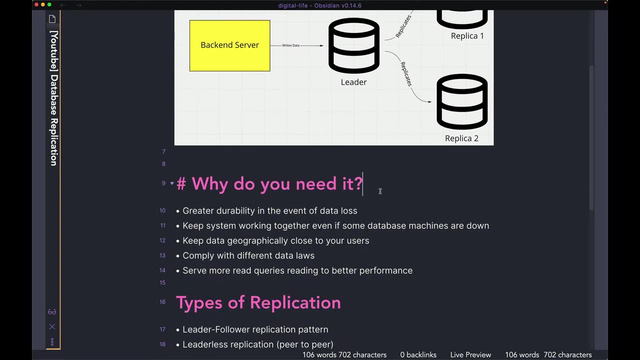 which, in this case, is replica one and replica two. Okay, So let's see. why do you wanna replicate the data? Because, of course, if you have a very popular application, your database can be petabytes and petabytes of data. And if you're replicating- 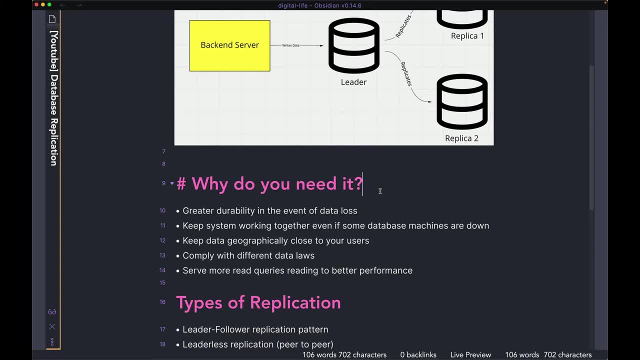 in multiple machines, then, of course, you will need to pay for both the storage and compute, so there must be a good reason that you are duplicating the data across different machines. so let's take a look at what are the benefits that you're getting. the first one is greater durability in the event. 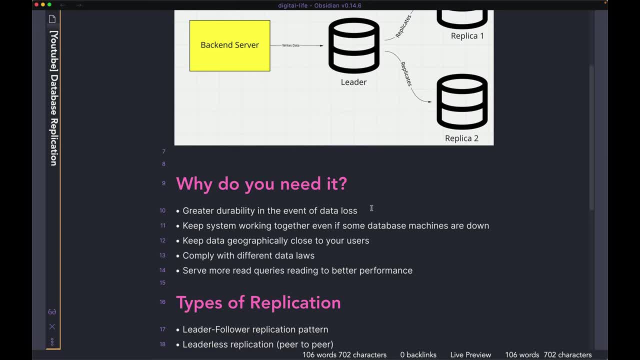 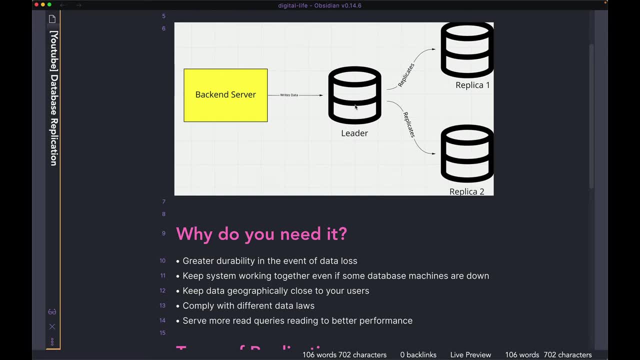 of data loss. this means that if there is any natural disaster or mechanical failure- so let's say that your leader node over here- for some reason the machine maybe catches on fire or there's just some random fault and the machine stops working- you still have all your data safe. 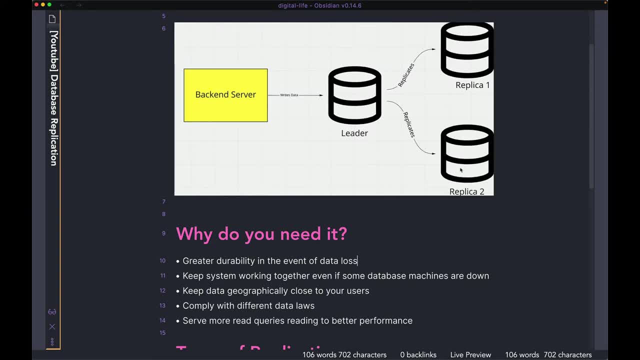 in replica 1 and replica 2. this is what I mean by. it gives you greater durability so in case of unforeseen situations like a hardware failure, you can rest in peace knowing that your data is replicated in different machines. the next one I have is keep system working together, even if some database machines are. 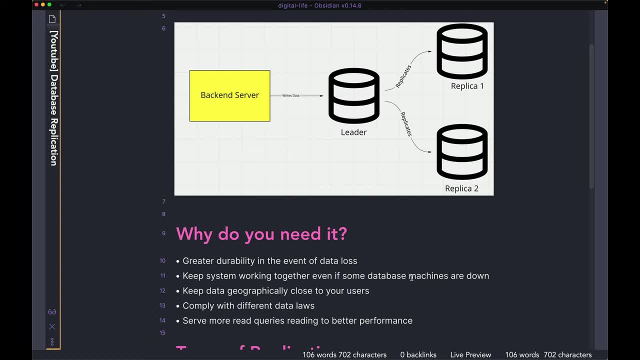 down. this is very similar to the first one, where if you have the same data in three or more different machines, then even if one of the machine is down, you can keep your app working by serving the data from your other machines. the next one is keep data geographically closed. 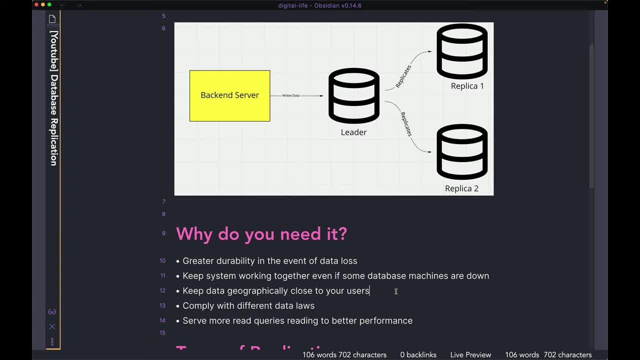 to your users, let's say: let's say you have a global application and you have users all across the world. so you have users in North America, you have users in Asia, Africa, Europe and the Middle East, right? so of course that means if a user from the Middle East signs into your application, 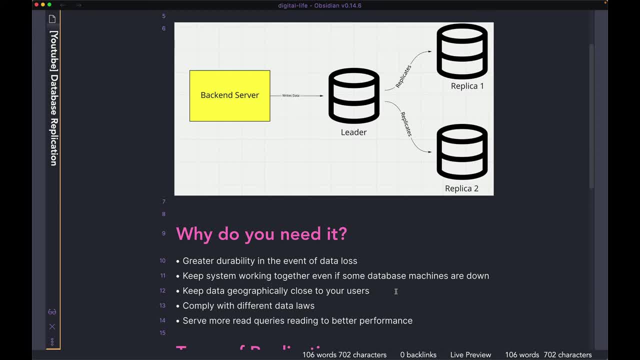 if you keep the data only in North America, that means whenever a user in the Middle East or Asia goes to your app, this data will have to be sent all the way across the Atlantic or Pacific to a entirely different place, just for the user to see their 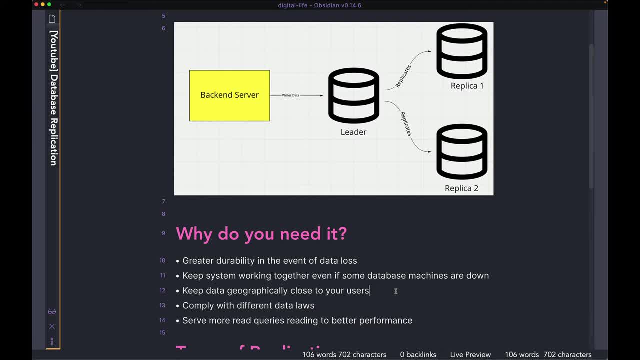 data. this can, of course, be very time consuming, because the data has to physically travel across the oceans and land and everything right, and of course this takes this takes a lot of time. so to avoid that, what you can do is you can keep the same data in multiple different locations. so 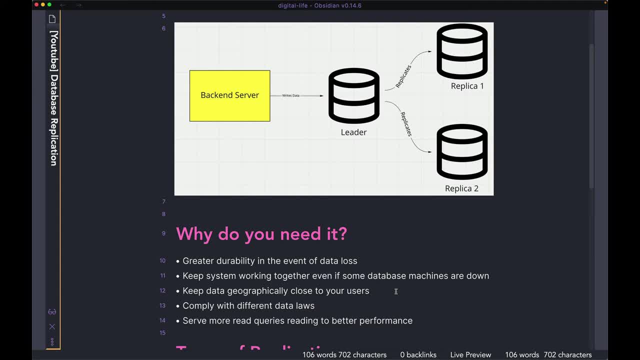 let's say you're keeping the user's data in Africa, North America, Asia and Europe. in this case, no matter where your user is and no matter where they sign in to your app from, the data can be served from the database closest to them. this means that no matter where they are, they're going to get a. 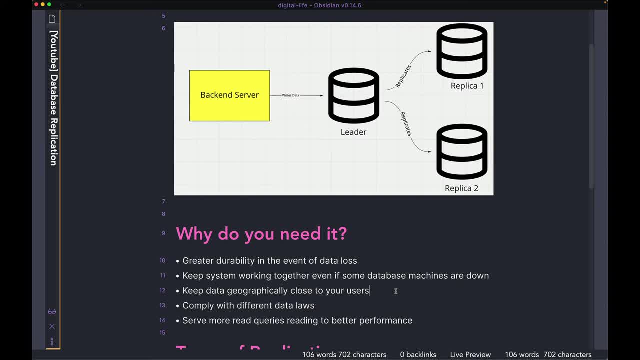 very good experience, because the data is not gonna travel across all around the world just to reach the user. the next one I have is comply with different data laws. so, uh, most countries have, or even like continents have- different data privacy laws that companies have to comply with. 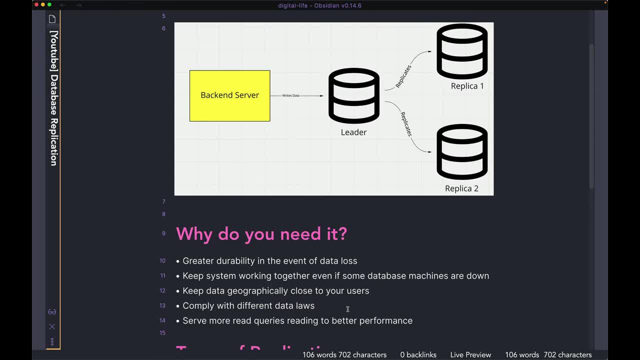 so Europe has some very strict data privacy laws of. California has somewhat some strict laws and even, like the rest of America, has some data privacy laws too. so, depending on where you're keeping your users data, you might need to comply with different data privacy laws and policies. so it's a good, it's a good idea to keep the data in. 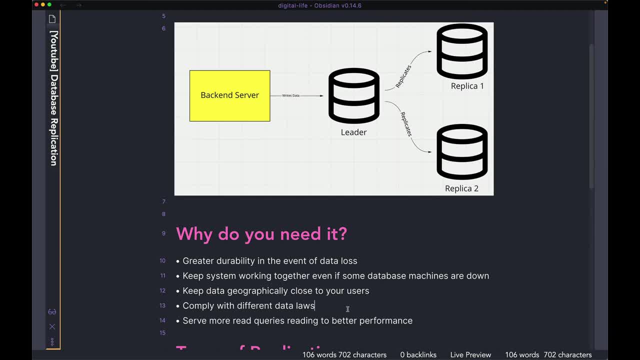 places and treat them differently so that, no matter where the data is, you are abiding by the different laws. so, yeah, you can see like the same data being replicated in different uh continents or locations just to comply with different laws correctly. the last one I have here is serve more read queries: reading to better performance. it. 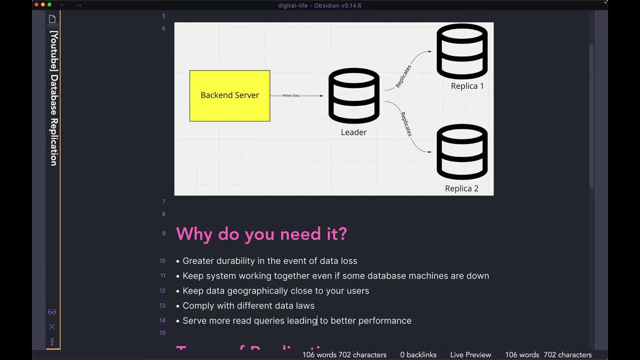 should be leading to better performance. there you go, so serve more read queries leading to better performance. what this means is, let's say that at 2 pm, every day, you have x amount of traffic coming to your application, and now, at 7 pm, every single day, you have a. 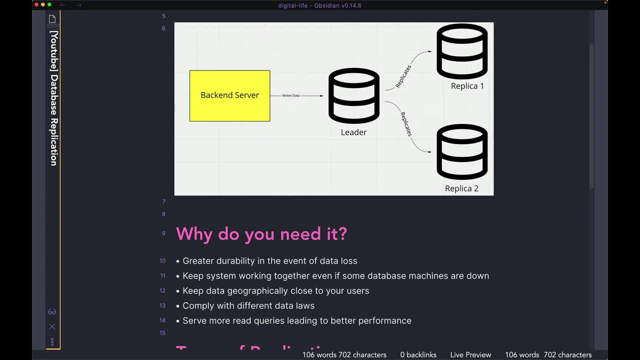 significantly higher load of traffic in your application. a higher load of traffic means, of course, more database queries. now, if you have your data in more than one machine, now during the peak hours, instead of that one machine being responsible for all the queries, you can use all your replicas, so in this case, all three of the databases which have the same data right. 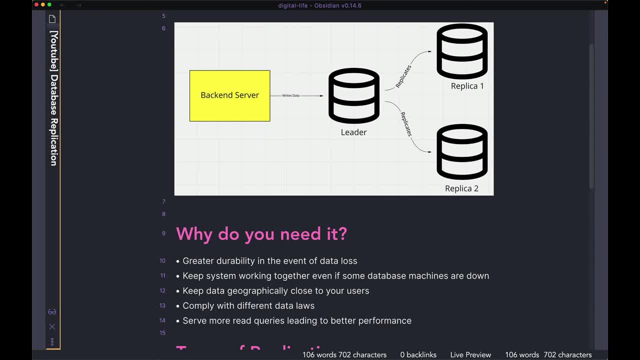 so what this is going to do is distribute your applications load across the three database machines, which of course means that each machine by themselves won't have to do too much work, and by doing so, what you're doing is giving your users a better experience, because if you had only 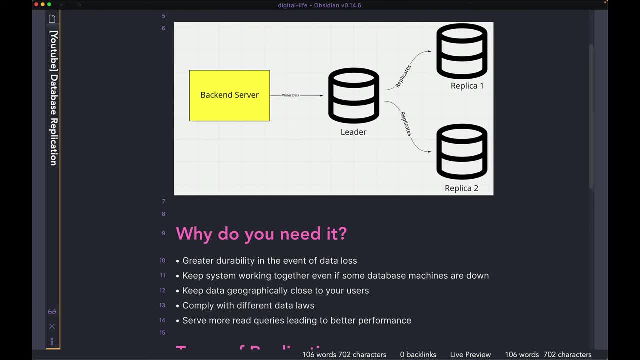 one database machine serving all the requests. during peak hour that means each of the request is going to take longer to respond and the users would have to be waiting for longer amount of time. so by serving the read queries from all the different replicas that you have, you're gonna 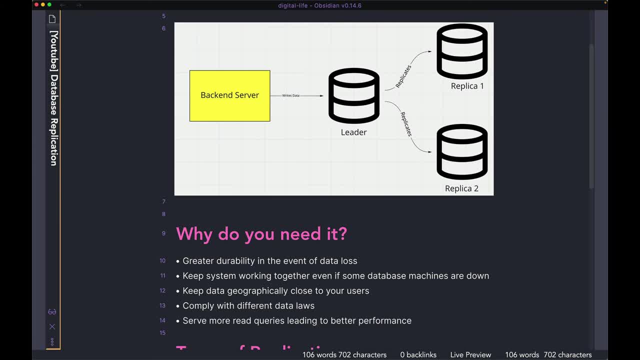 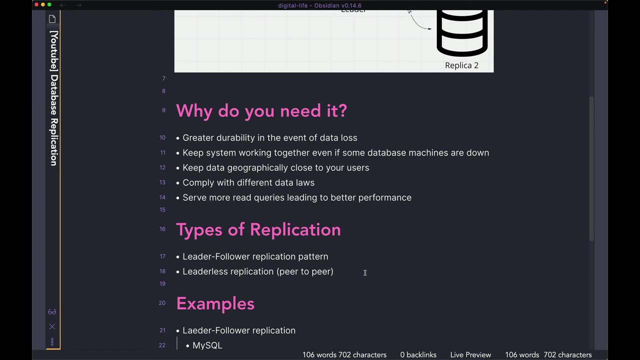 be reducing the workload and you're going to be reducing the load of traffic load on each of the machine, leading to a much better user experience for your users during these peak traffic hours. all right, so those were some of the benefits, and now let's talk about the different types of replication. over here, I'm just gonna talk about the two different. 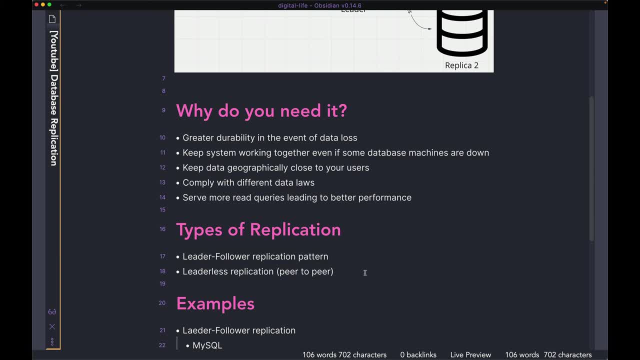 kinds and very high level. but I think I have two more videos coming in the next week or two where we are gonna dive deeper into each of these and go through how they actually work. so the first one I have here is called leader follower replication pattern. this is a very, very common pattern. 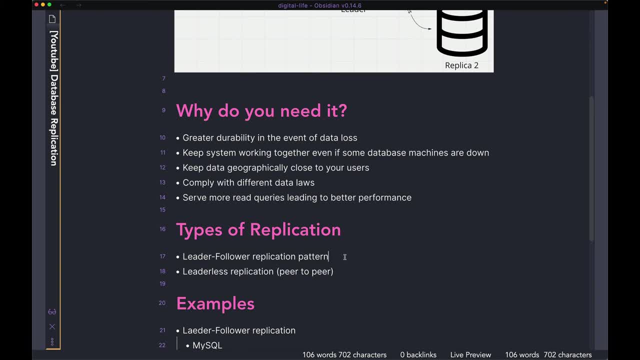 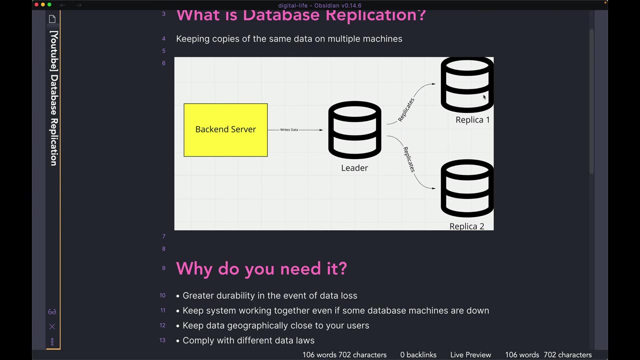 that companies use to replicate their data. this is especially common in relational databases. so the idea is very simple. you have a leader node and then you have a bunch of follower nodes. if you take a look over here, you have your leader and then you have your replica. all the rights go to. 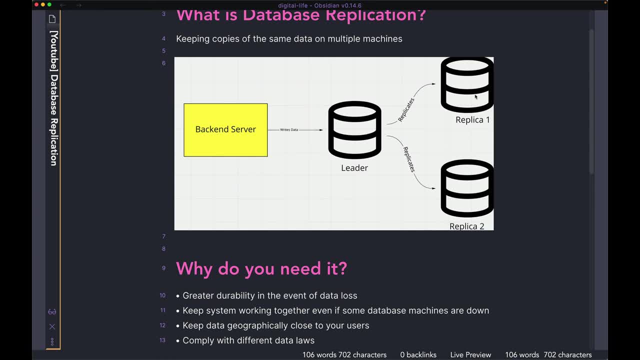 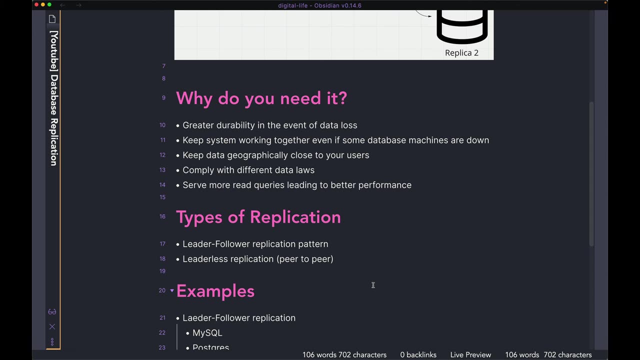 the leader and then the leader replicates the data data to all the follower machines, right, as I mentioned. I am going to go deeper into this system in one of the future videos, but for now just remember the name, okay. the next one is called a leaderless replication or a peer-to-peer. this is 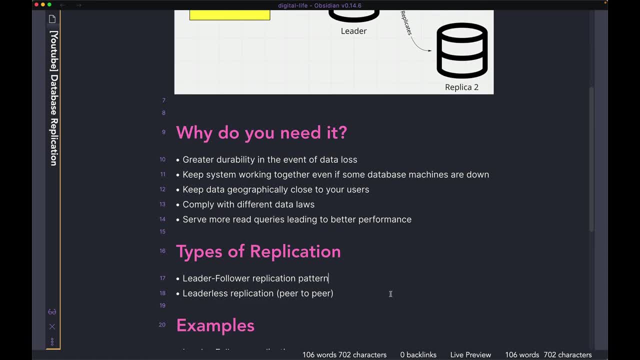 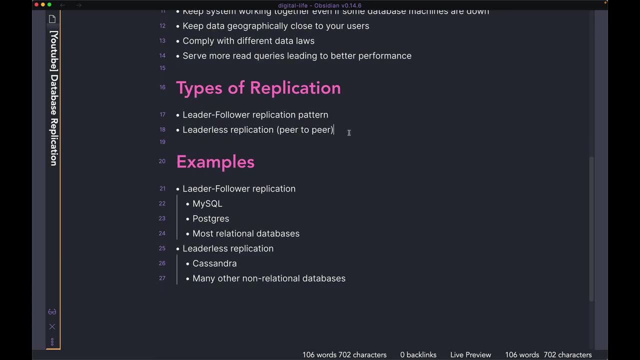 a very different model to what I just talked about, and this is more common in non-relational databases like Cassandra. okay, so I'm not going to go into too much details about either of these because I have individual videos coming up, coming up in the next weeks, where we go into the details of both of these. 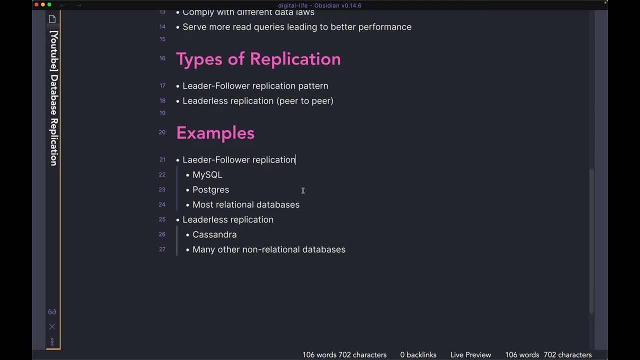 all right, so we're going to wrap up with some examples. for the leader follower replication, it's very common in relational databases like mysql and postgres. and for the leaderless replication, it's very common in non-relational databases like Cassandra. so yeah, hopefully this gives you somewhat of an idea of what database replication. 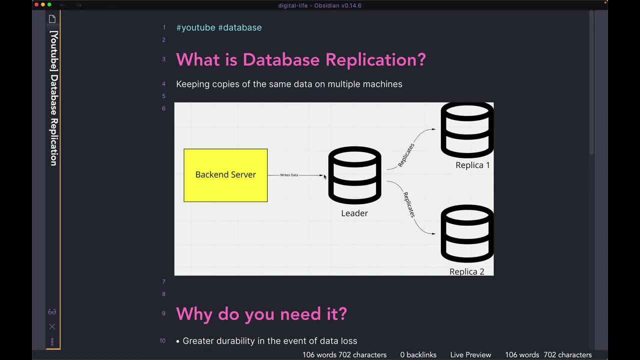 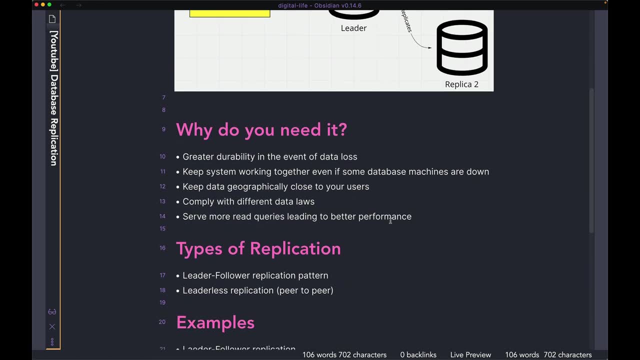 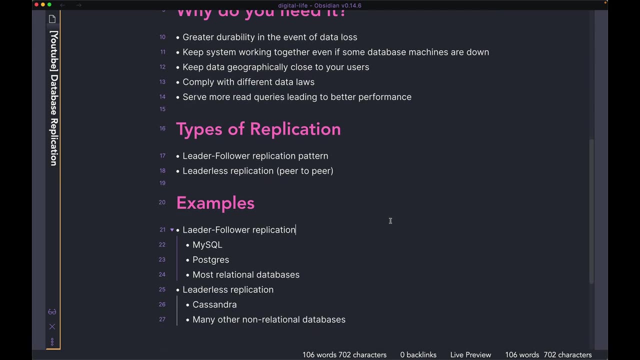 is and what benefits we get out of it. when it comes to how the replication actually happens, there's a lot of technical details behind it. that's what we're gonna dive deeper into in the next two to three videos, so stay tuned for those. if you have any questions about everything that I went through, please leave. 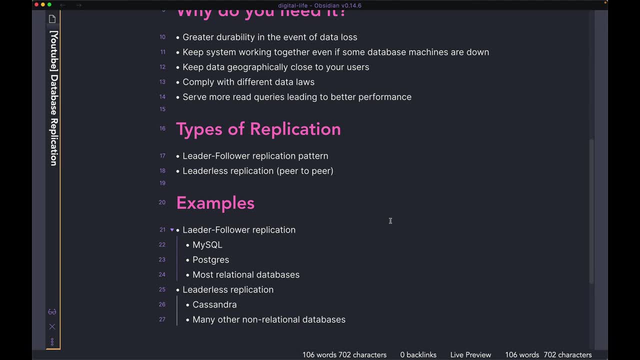 them in the comments and I'll and I'll get back to you as soon as I can. with that being said, I hope you guys have a good rest of the day and I'm gonna catch you guys in the next one. bye.